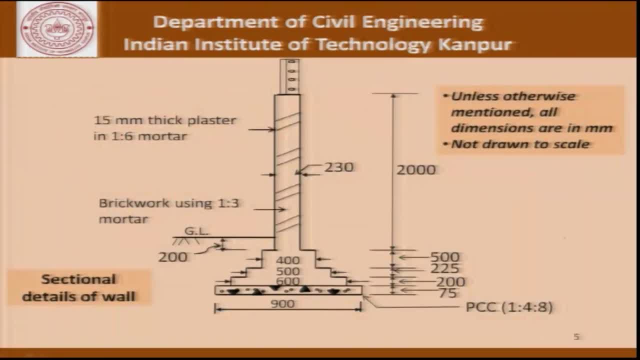 here centre to centre. Now, if we look at the details of this boundary wall, this was the section which was given that there is a ground level. there is a certain amount of excavation which has to be done. there will be brickwork using 1 is to 3 mortar. here there will be a 15 mm thick plaster. 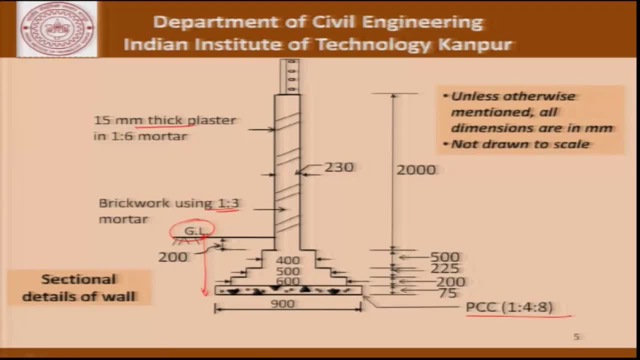 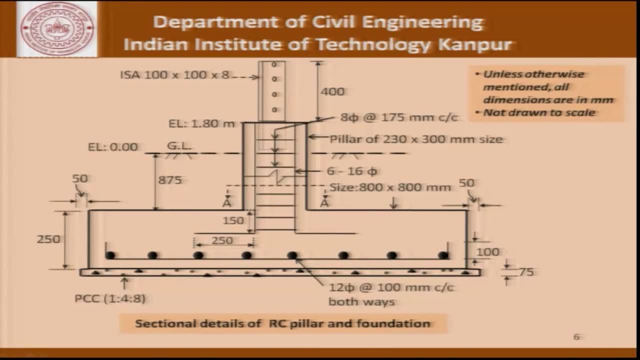 on both sides of the wall there will be PCC 1 is to 4 is to 8 at the bottom and as far as the RC pillars are Concerned. this is the details of the drawing that the reinforced concrete will be in the 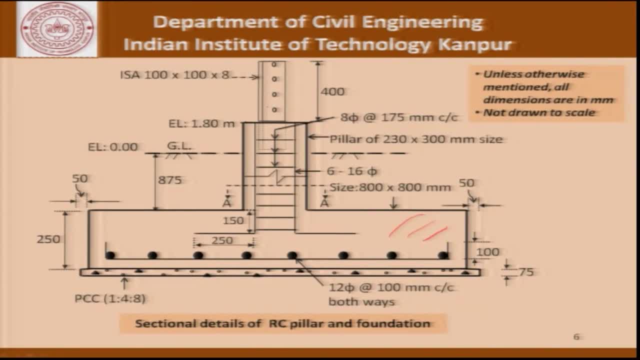 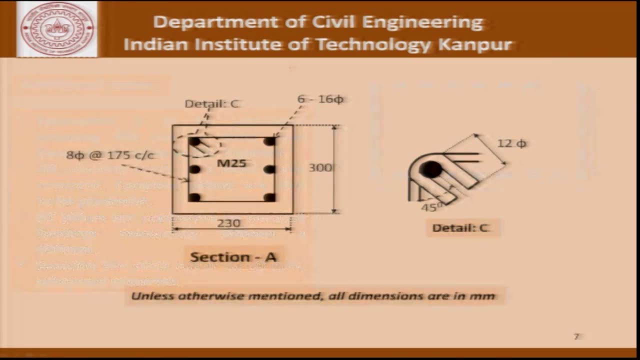 foundation and in the columns, and there will be an angle which will be fixed at each of these RC pillars. these are the places where the barbed wire will run. This picture here was used to explain what is the details of the stirrups involved. and then there were 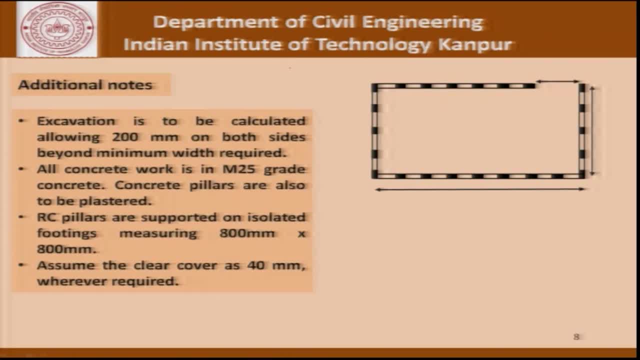 additional notes which were told to you, which said that excavation is to be calculated allowing 200 mm on both sides Beyond the minimum width required. all concrete work is in M25 grade concrete. RC pillars are supported in isolated footings. clear cover is for TMM original and final ground. 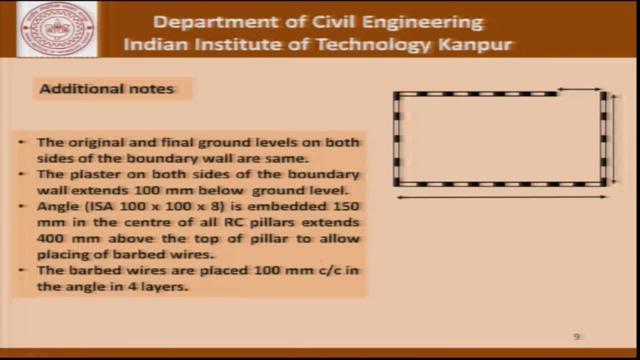 levels are the same. The plaster on both sides of the boundary wall extends 100 mm below the ground level and angles are embedded 150 mm in the centre of the RC pillar, extending 400 mm the top of the pillar to allow placing of barbed wires, and barbed wires are placed at 100 mm centre. 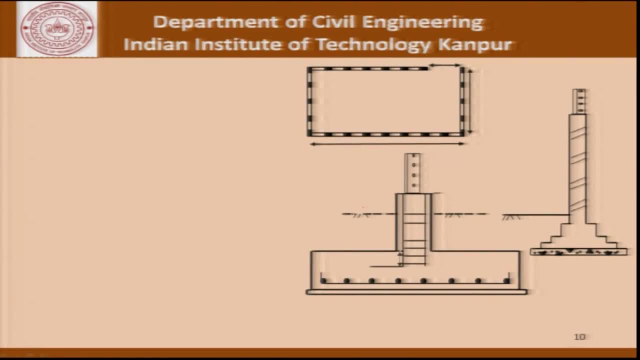 to centre in the angle. This is the part of the boundary wall that is needed to bring the concrete to its initial position. So further we can discuss how to identify the structural steel angles for a concrete structure and what are the rest of the structural steel angles. 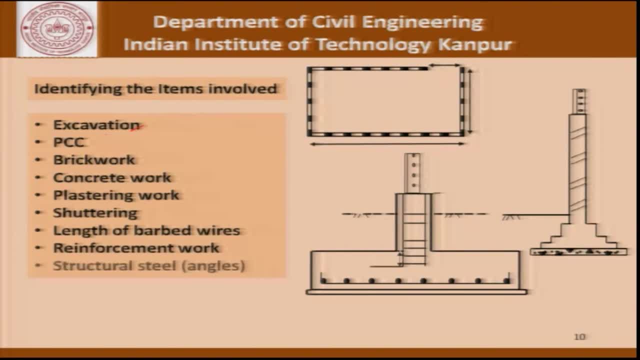 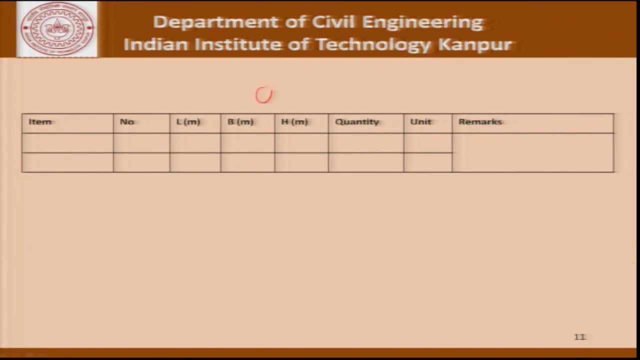 With this description of the boundary wall, we went about identifying the items for this particular project. We have excavation, PCC brickwork, concrete work, plastering work, shuttering work, length of the barbed wires, reinforcement work and, finally, structural steel angles. So this we had identified as the different items. Then we went into a detailed exercise to calculate the quantity of the concrete and then the next transformation process will be done. In this section we will discuss how we are 너fcile-neutral steel and what is the horizontal boundary wall property and what is the horizontal boundary wall property and the what is the horizontal boundary walls and what is the horizontal boundary wall property. 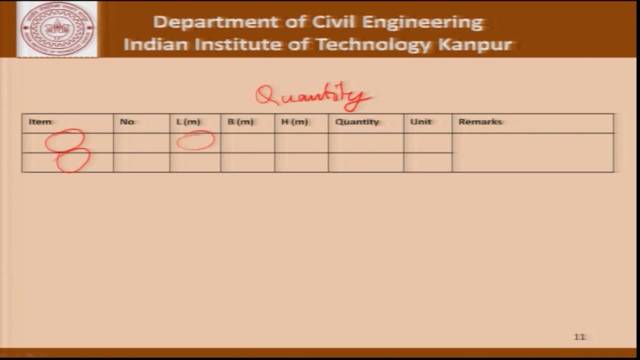 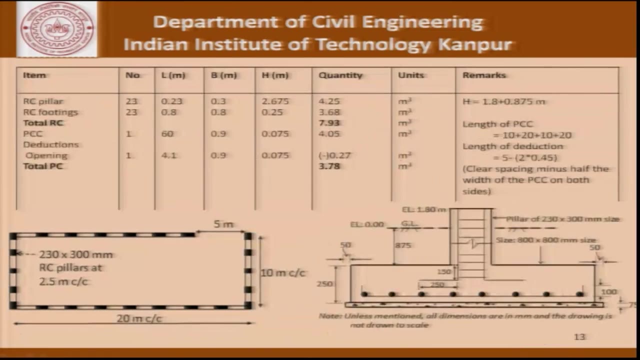 of the different items by using the concept of length, breadth, height and finally arriving at the quantity, sometimes its length and breadth. there is no height, whatever the units, and as an example, we calculated the total quantity of earth work involved as 87.83 cubic meters. 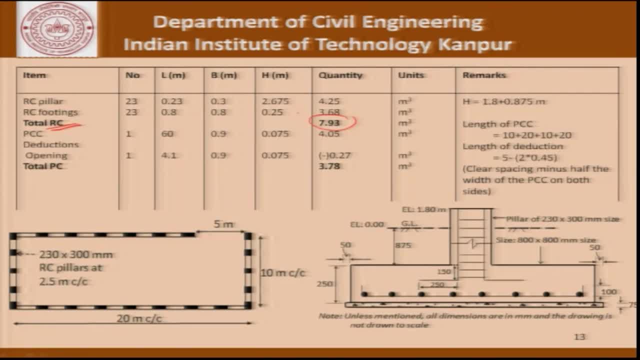 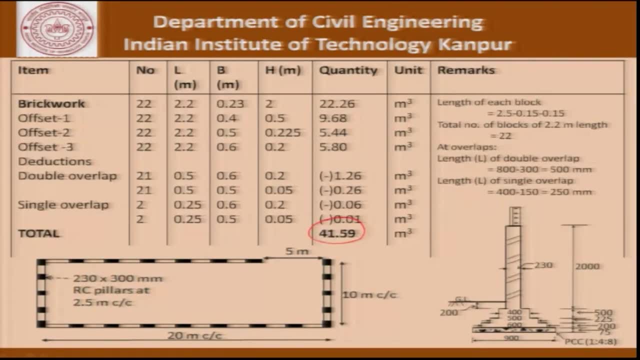 the quantity of reinforced concrete to be 7.9, the total quantity of pcc to be 3.78 cubic meters, and so on. brick work, similarly, was calculated as 41.59.. Once we have completed this exercise, what happens is that we have a description of the 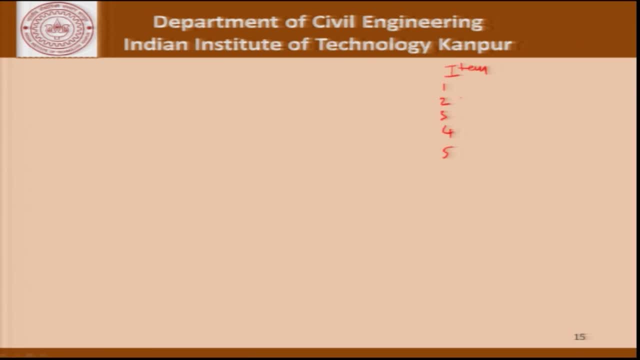 items 1,, 2,, 3,, 4, whatever they are in this case excavation, pcc, brick work and so on. we find, then, the rates from a standard source- it could be the daily schedule of rates or any such known set of rates or our own numbers that we may have- and based on this rate for 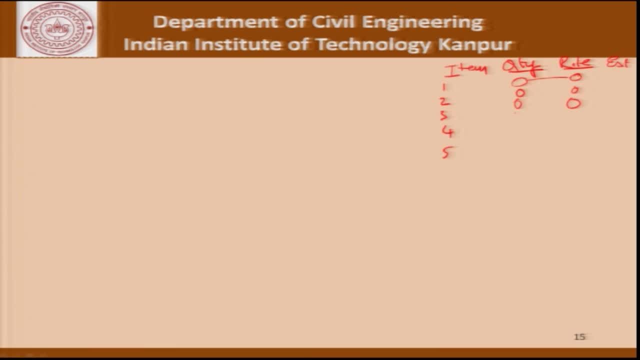 each of these items, We get the estimated cost for each of these items and once we have this, if we add up this number here in this column, we will get what we will call as the estimated cost of this project. Once this is completed, then we declare to the contractors- and that is what we did- this: 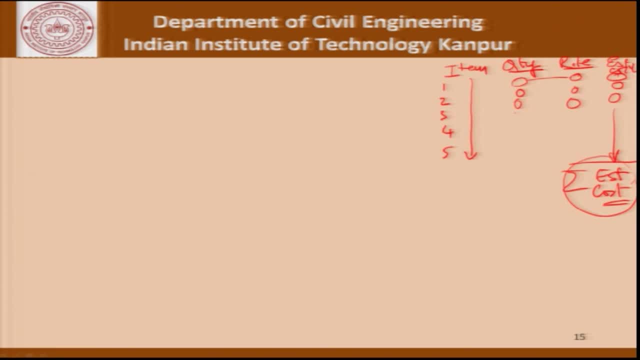 time. in our example, we said that these are the items of work, these are the quantities involved. this is the estimated cost of the project. now you please let us know at what rate will you be willing to execute this project Now, when this exercise goes to the next step? the contractors know this number and contractor. 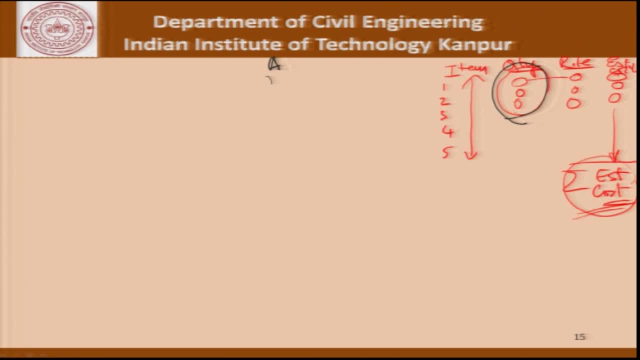 A will say that my rate, which is R 1 for this item, R 2 for this item, R 3 for this item, and the total rate that the contractor A codes, the total amount that the contractor A codes, let us say, becomes C: A. So this is the cost at which contractor A is willing to do the 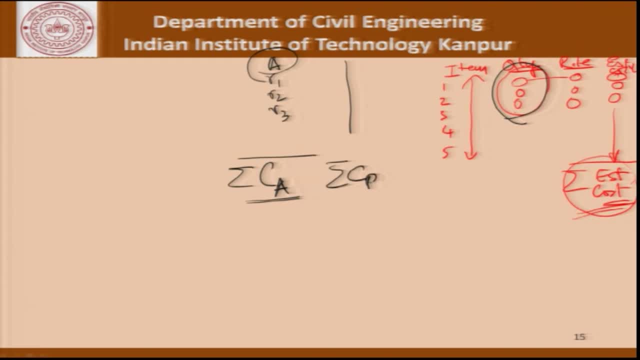 work. similarly, we can have an exercise here and we will come up with the cost that contractor B wants to do it. these costs obviously need not be the same as the estimated cost, because each of these contractors will have different rates and so on. the quantities remain fixed. 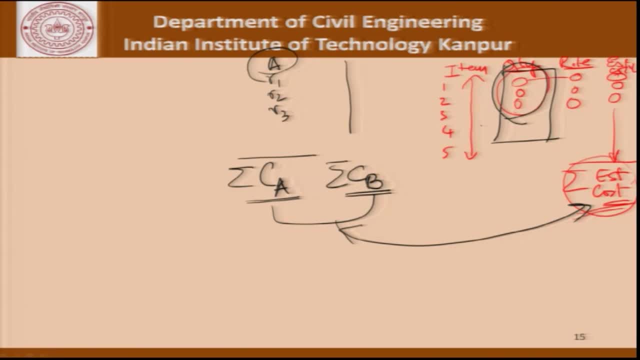 because these are something which we have already estimated from our drawings. having carried out this exercise, now we can decide which contractor do we want to give it to. let us say, we give it to the contractor B. So now we have an estimated value, which was earlier. we have a contract value which. 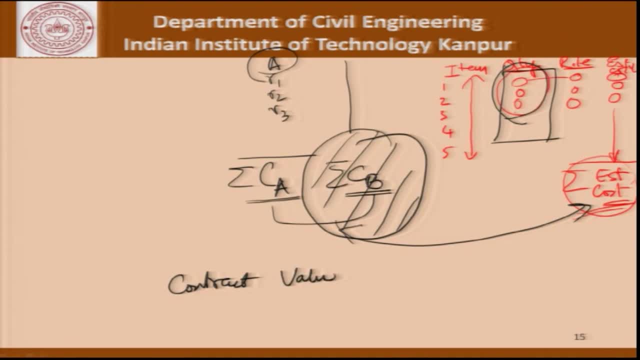 is the cost at which this contract has been awarded. let us say C, B. then we went through examples of running account bills where the different quantities of work, that is, we have items 1, 2, 3 and 4, 5, whatever they are. we have date one, we have another date at this date. 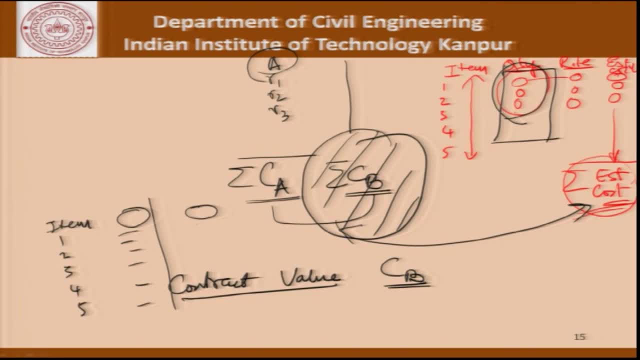 what are the different items that have been completed, to what extent? and at the next date, what are the items which have been completed till that date? We went through the exercise of calculating the value of the work done at this point in time- value of the work done at this point in time- and decided and found out how much. 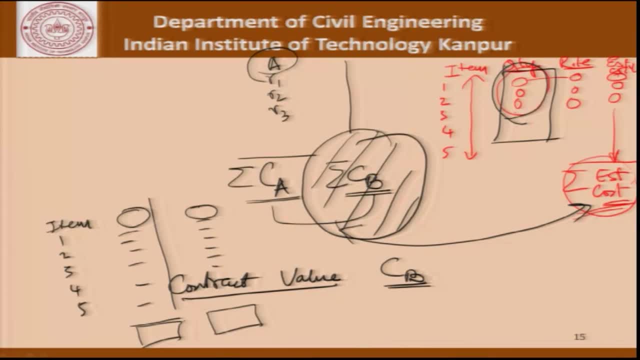 is the money payable to the contractors at different points in time, based on these rates, which were quoted by the contractor and accepted by us as clients, and the quantities of work which have been done at different points in time. So with this background, which is just a recapitulation of what we have already done, we will now 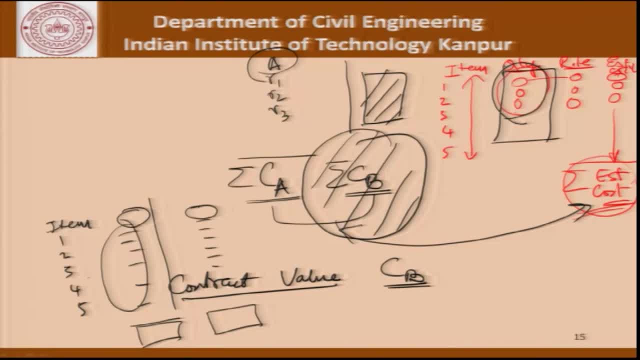 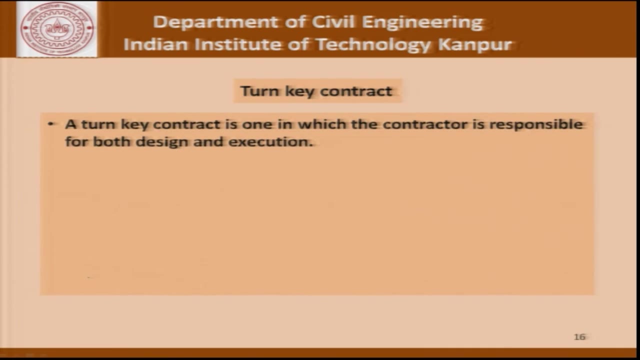 try to examine what are the different other options that we had as far as executing this contract is concerned from the point of view of payments. The first thing that we want to do is to discuss the turnkey contract. A turnkey contract is one in which the contractor is responsible for both design. 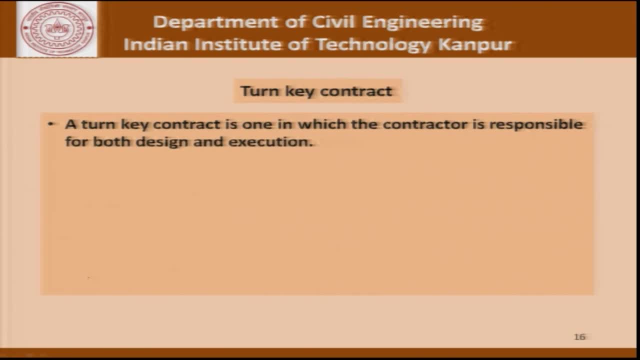 and execution, that is, the client does not do the design, The owner or the client obviously still provides the functional requirements and approves the design and the drawings. So in our example- a small example, of course the client will say that well, I want to fence. 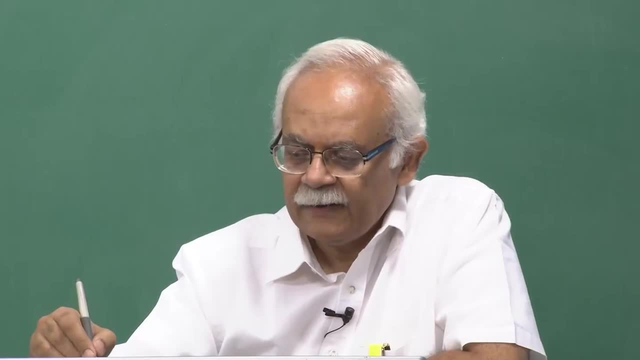 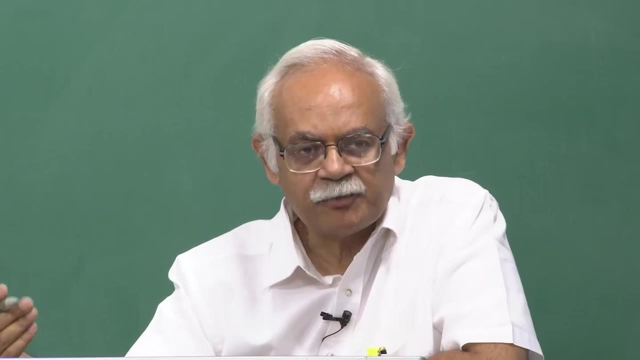 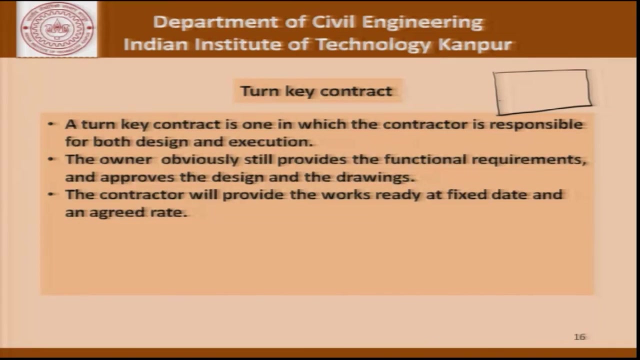 this area, which may measure some x by y, and it is left to the contractor to come up with the drawings. Those drawings and the design are approved by the client and then we move on to design the payments. The contractor will provide the works ready at a fixed date, at an agreed rate. 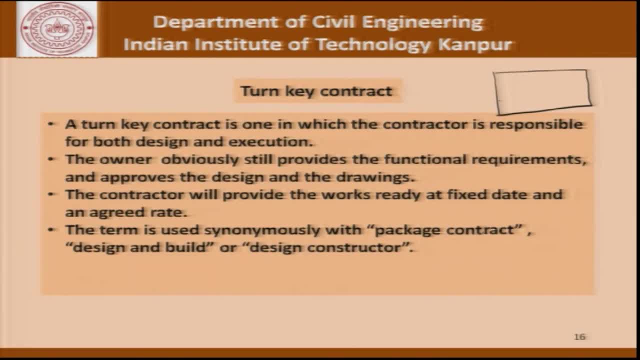 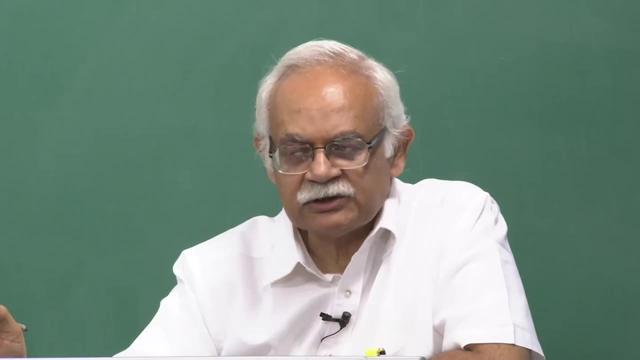 The term is used synonymously with the package contract design and build or design constructor, and is also known as EPC contracts, which is engineering, procurement and construction. So the contractor does the entire design, gets the approvals from the client and proceeds to execute the project, and it is agreed upon between the client and the contractor. 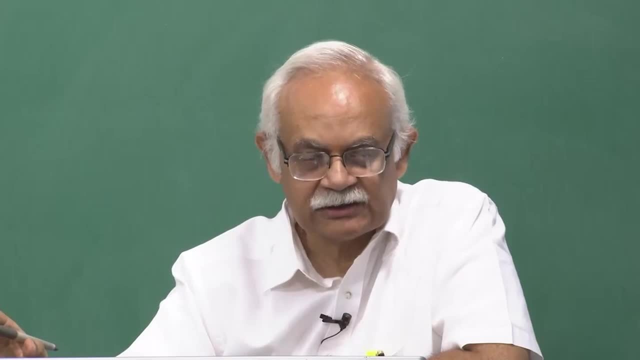 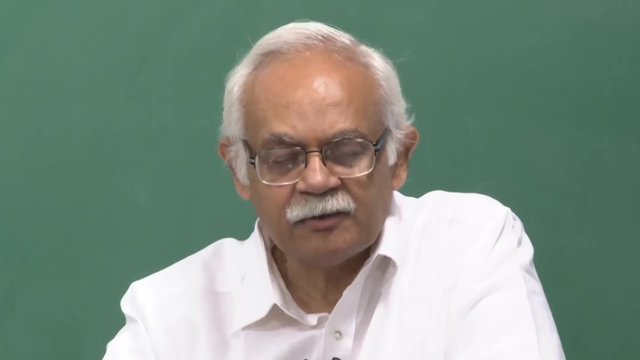 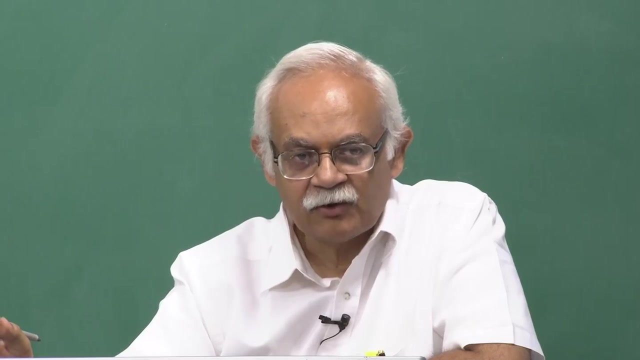 That well, this is the total cost of the project As far as the client is concerned. there is no cost incurred in designing. there is no cost incurred in determining the different quantities, the different rates. none of that is involved and it is all left to the contractor who does the drawings, who calculates his 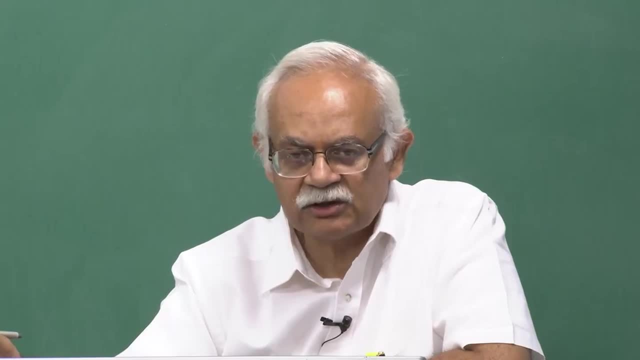 own quantities, comes up with the rates, comes up with the total cost. Of course, the client has to be very clear in its mind that how they will evaluate different proposals. Different contractors will obviously come up with different kinds of boundary walls perhaps, and the client should know how to evaluate it. 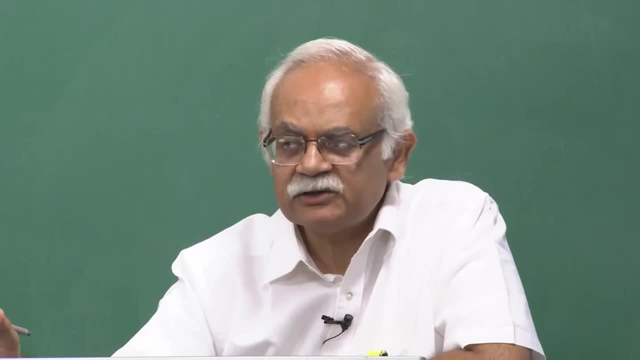 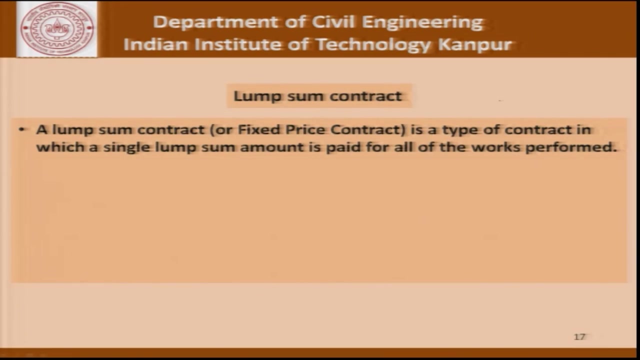 But, having said that, the turnkey project has its own advantages, because it saves the client of a lot of detailed engineering, which they may or may not have the capability to do, sometimes Coming to what is called a lump sum contract. this is a type of contract in which a single 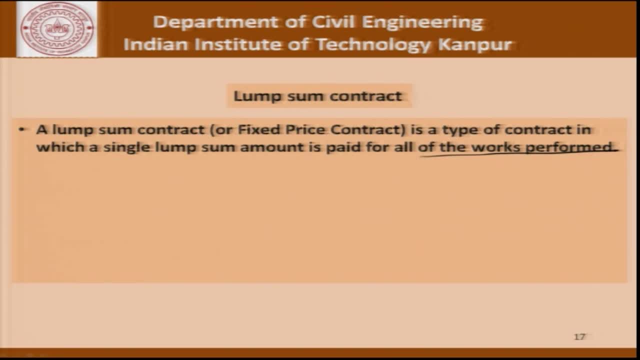 lump sum amount is paid for all the works performed. All the works performed may or may not increase. All the works performed may or may not include the design and the preparation of drawings and the detailing. So for example, in our case we can still give the drawings and say that well there. 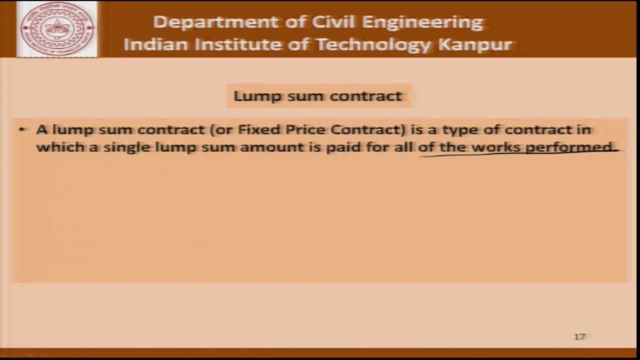 are no items and their rates are yours, and the contractor works out a total value itself and submits the contract and therefore, even at the time of running account bills, we do not have to measure the quantities of the different items In this contract. the contractor is responsible for completing the project within the agreed. 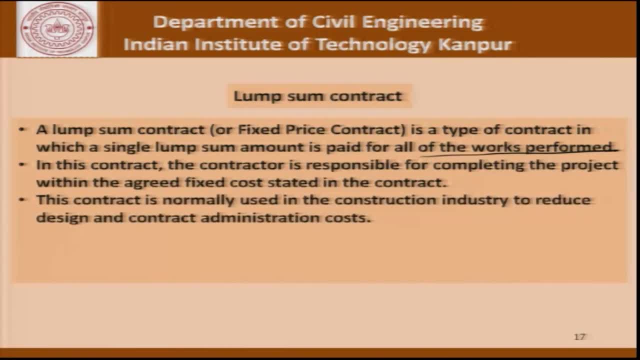 amount- Fixed cost- is stated in the contract. This contract is normally used in the construction industry to reduce the design and contract administration and is simple to administer, most suited for simple and small projects where the project is already well defined and changes are unlikely. 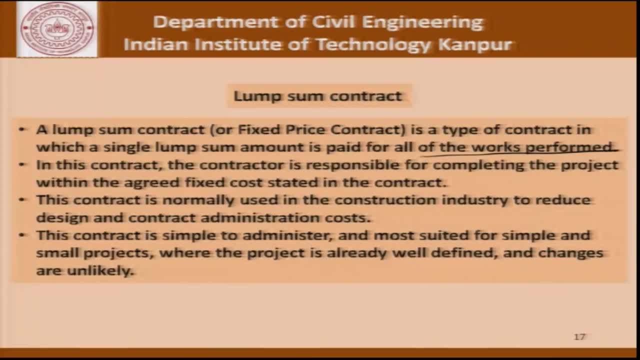 So if the boundary wall, for example, what we are talking about is clearly known, it is a simple example where anybody can calculate the quantities. you just have to give the drawings, The contractor can work out the details, can submit a fixed cost at which that contractor 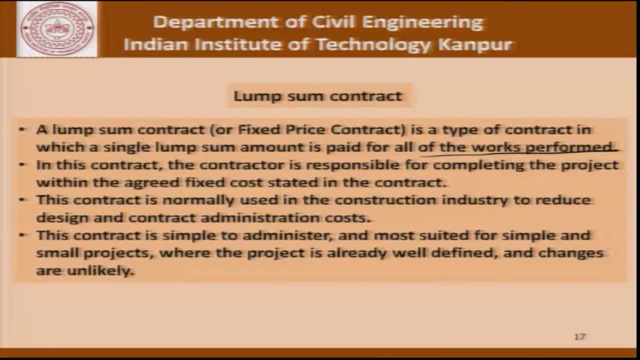 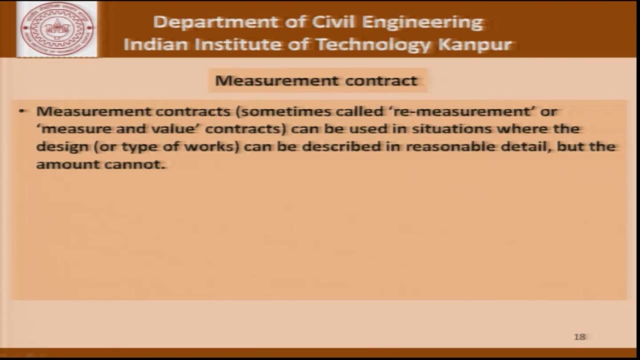 is willing to execute the job. So for small projects where the situation is fairly clear and not likely to change at the word go even before the work has to be started, these contracts can be recommended for adoption. As far as measurement contracts are concerned, they are also sometimes called re-measurement. 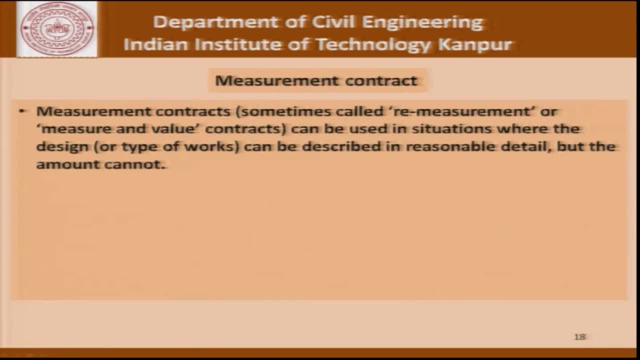 or measure and value contracts. These are situations where the design or the type of work can be described in reasonable detail, but the amount cannot be, And measurement contracts can allow an early start on the site before the design is complete, and they can allow changes to be made to the works relatively easily. 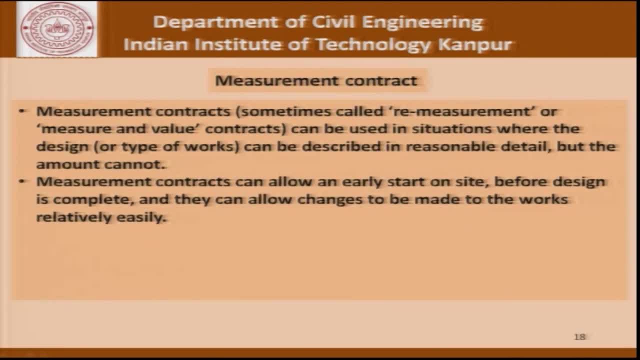 So, for example, even in the case of the boundary wall, we may not have worked out the final details of the depth of the angle embedment or the length of the angle projection above the boundary wall. allow the contractor to proceed with the excavation and the PCC work, and that is what is being. 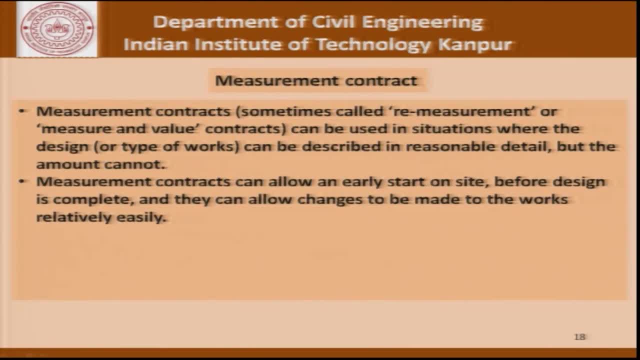 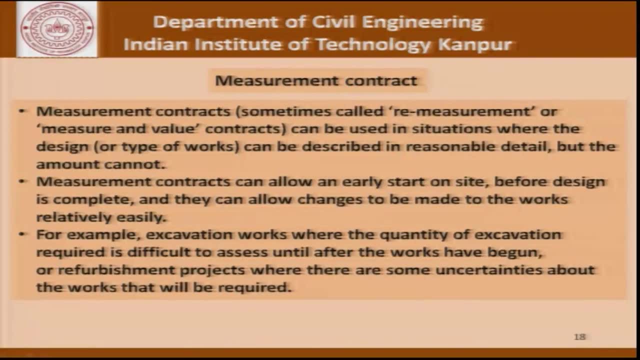 said here that the work can be started even before the complete design has been carried out. that is what stated here. the excavation work, where the quantity of excavation required is difficult to assess until after the works have begun, or refurbishment projects, where there can be some uncertainties about the work that will be required. these contracts: 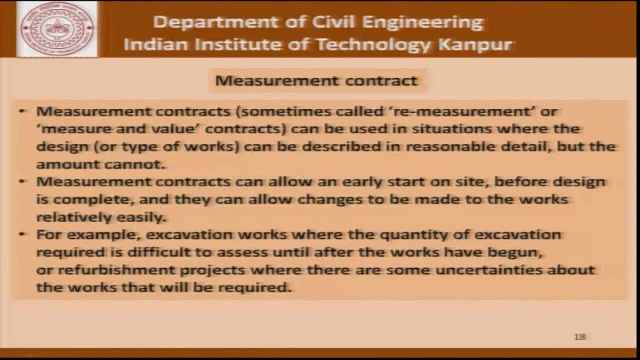 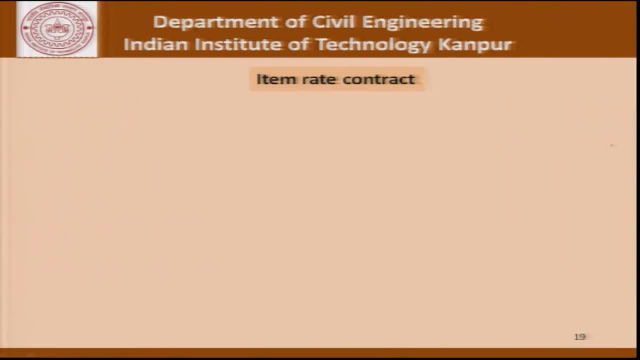 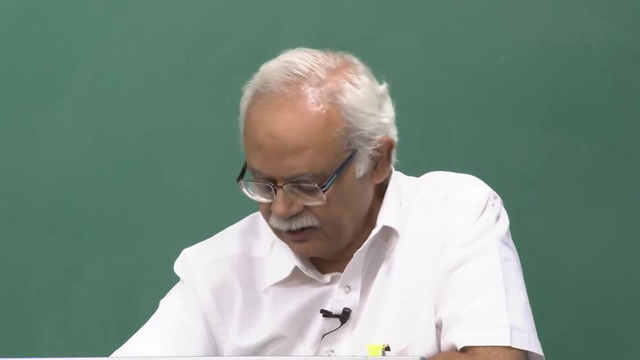 are recommended, because what we have to do is to take the measurements and pay the contractor for the actual work carried out. now, as we said, there are three variations of this measurement contracts. let us talk of the item rate contract, and that is, in fact, the contract that we have. 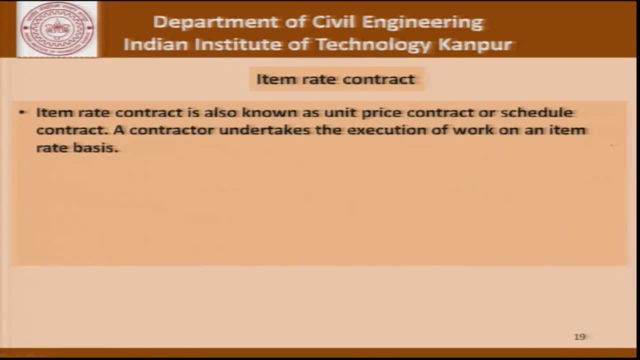 discussed in detail. the item rate contract is also known as the unit price contract or schedule contract. a contractor undertakes the execution of work on an item rate basis, so the items are known and the rates are quoted and that becomes the basis to determine the contract value. the 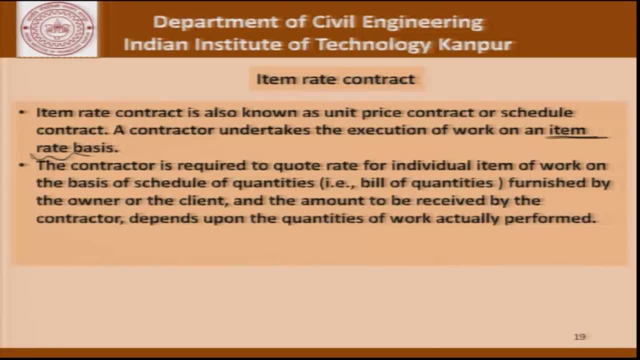 contract is required to quote the rate for individual items of work on the basis of the schedule of quantities- the bill of quantities, that's what we talked about- furnished by the owner of the client, and the amount to be received by the contractor depends on the quantities of 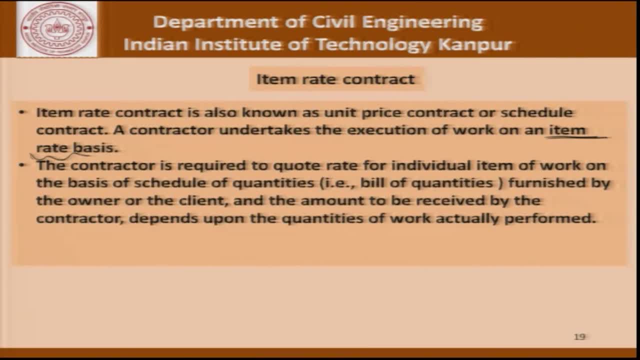 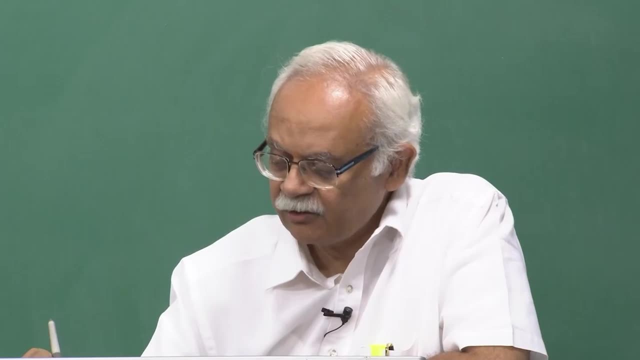 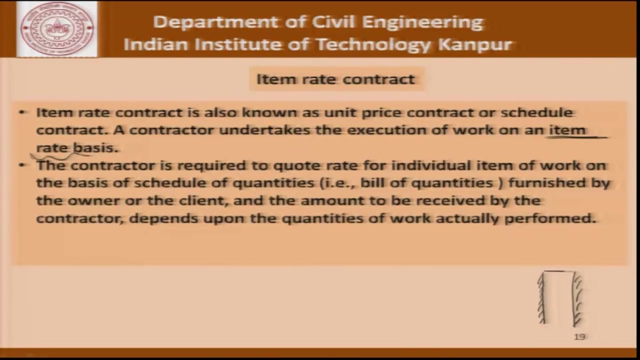 the work actually performed. so therefore, if you recall, the quantities of work actually performed may or may not be exactly the quantities of the work that were planned or estimated. you would recall from an example that when we calculated the plasters- and I have addressed this before also- we talked of the quantities of plaster on the walls and we had not calculated. 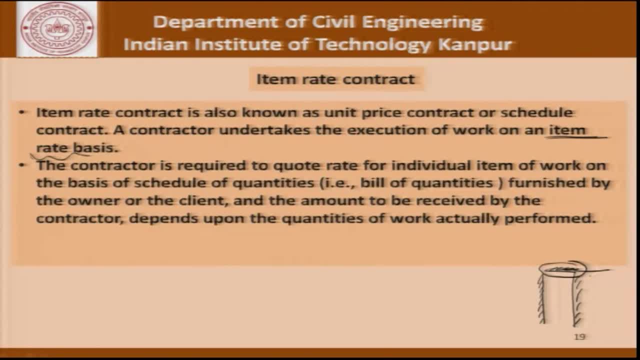 the quantity of plaster on the top of the wall, so there will be a deviation as far as quantities are concerned. this kind of contract allows us to handle that kind of deviation without any trouble, except that of course we must remember that these deviations should not be large in. 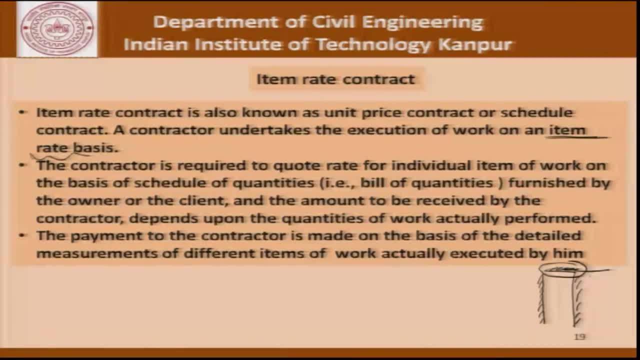 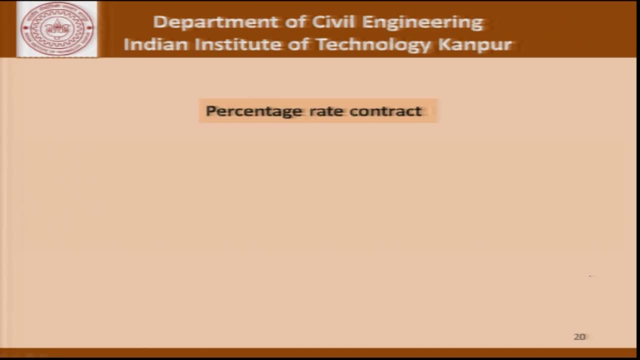 magnitude payment to the contractors made on the basis of the detailed measurements of different items of work actually executed by him. then we come to percentage rate contracts. in this case the client or the owner draws up the item rate tender, the bill of quantities, in the total amount. so what we have done, 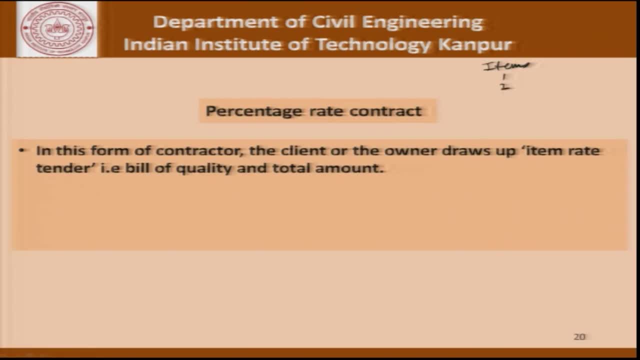 is that for the different items- one, two, three, four- we know the quantities of these items. the owner draws this up and also the rates. so we have these rates and we have therefore an estimated cost. once we have this estimated cost, we ask the contractors or bidders to submit a bid as to whether they are willing to do. 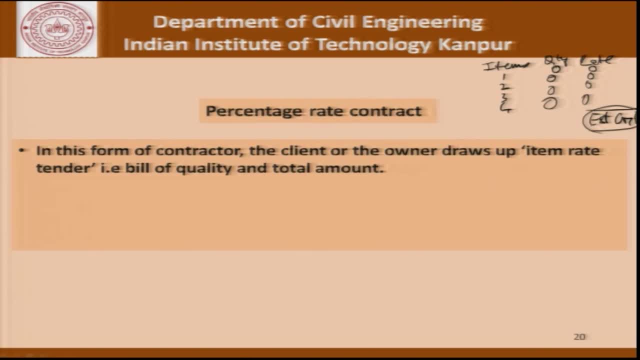 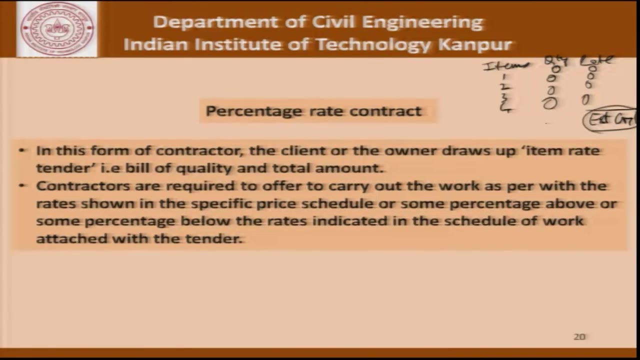 the work at a rate, at an amount which is higher or lower than this estimated cost in terms of particular cost. So the percentage is, that is, contractors are required to offer or to carry out the work as per the rates shown in the specific price schedule, or some percentage. 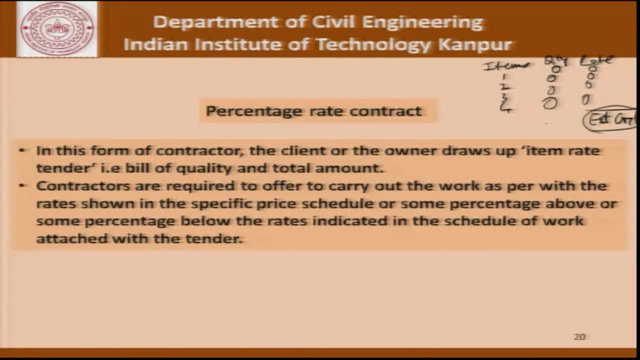 above, or some percentage below, the rates indicated in the schedule of work attached with the tender. So what the contractor submits is a number which is may be plus 10 percent or minus 5 percent of the estimated value. So if the estimated value is, let us say, 100.. 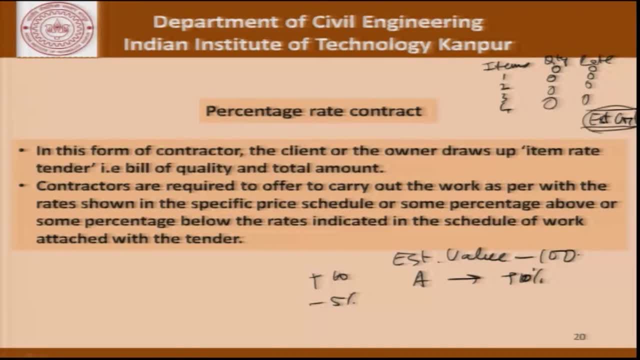 Contractor a submits plus 10 percent of this value. contractor b submits minus 2 percent of this value. basically, what is being said is that this guy is willing to do the work at 98 and this company is going to charge 110 to carry out the work. The difference? 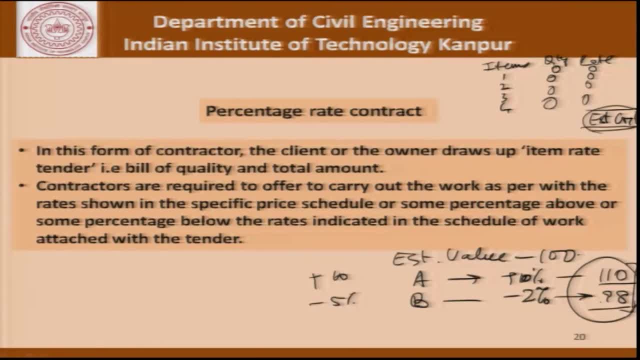 between now. in this case, if you compare this discussion with the item rate contract, the contractors or the bidders had the freedom freedom in that case. in the item rate contract, the bidders had the freedom to choose their rates. So company A could come up with a total of 110 by varying the rates of the different. 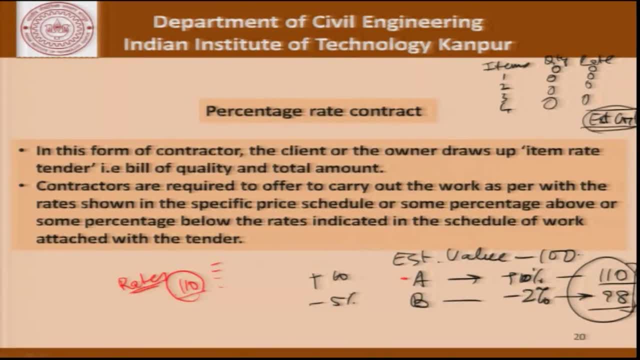 items. Company B could come up with 98 by varying the rates, But in this case the rate remains fixed and the total amount that they have quoted here, which is plus 10 percent or minus 2 percent, that is distributed across the board. This has implications in terms 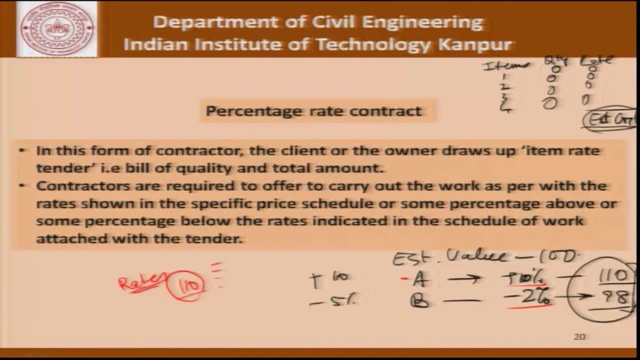 of understanding of front loading of contracts, And that is something which I am leaving to you to think and understand how front loading can be avoided through percentage rate contracts. We must also remember that, as far as large projects are concerned, when we are talking of civil contracts, the single large contract- electrical works in the same project- is another. 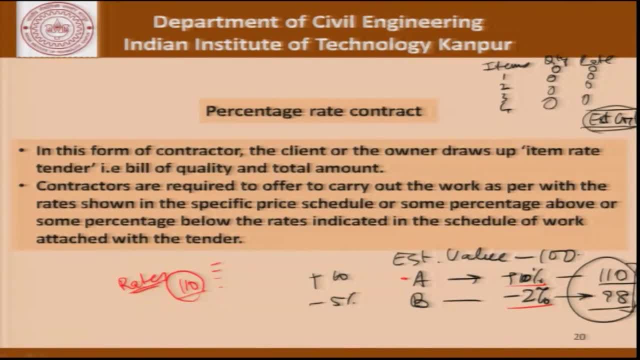 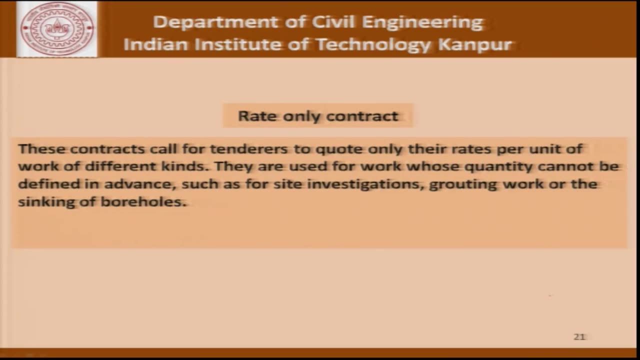 large contract So we could operate percentage rate contracts, and this also does not require, with this discussed on the percentage rate contract, as contrasted to the item rate contract, The third variety here is the rate only contract. Now, in this case, the contracts call for tenderers to 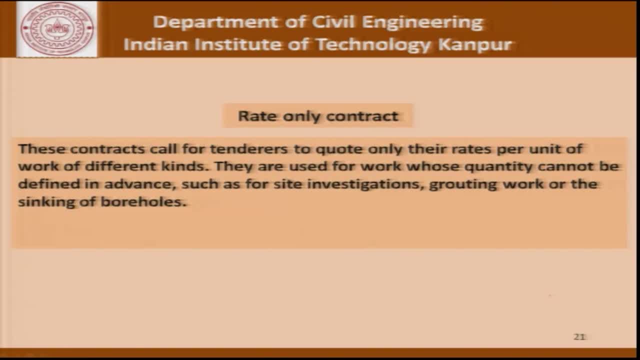 quote only their rates per unit quantity of the different works involved. They are used for work whose quantity cannot be defined in advance, such as for site investigations, grouting work or sinking of boreholes. So in this case it is a measurement contract, that is, the payment will be made based on. 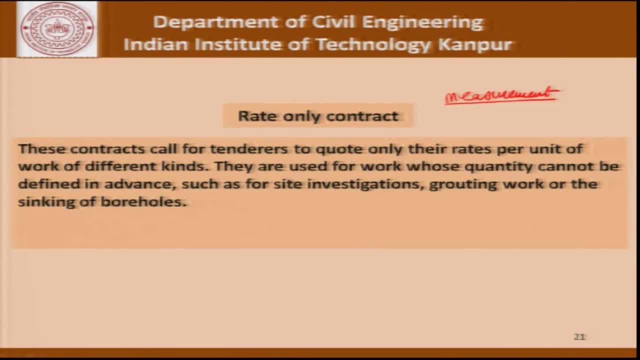 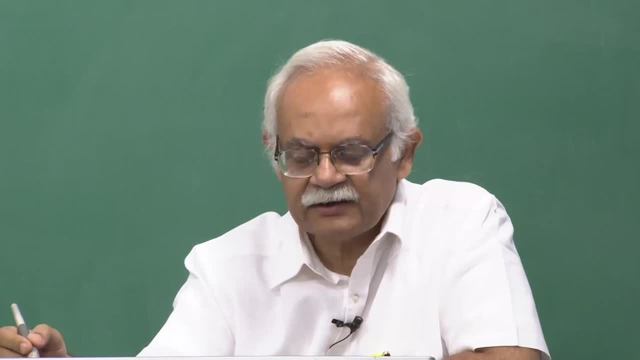 the measurement of work carried out for different items, whether it is excavation or plaster or whatever it is. but the quantity is not given. So the contractors submit only the rate and, depending on the actual measurement of the work carried out, the payment is made. 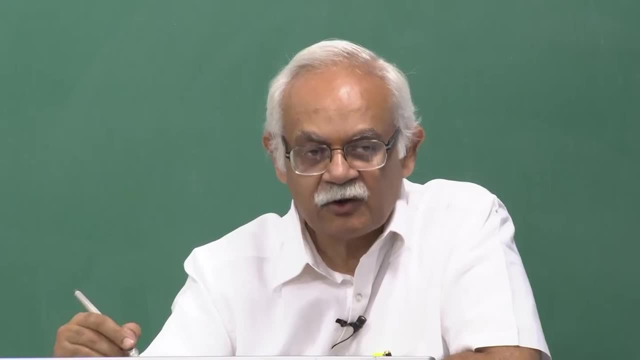 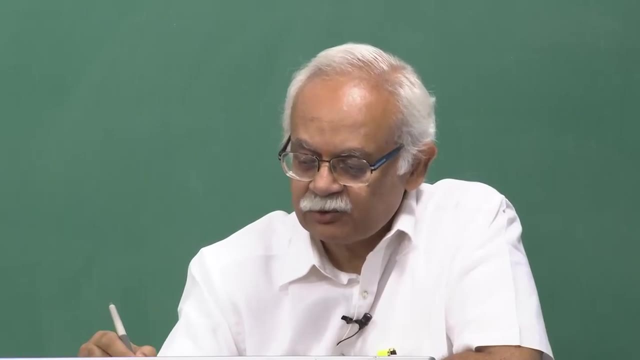 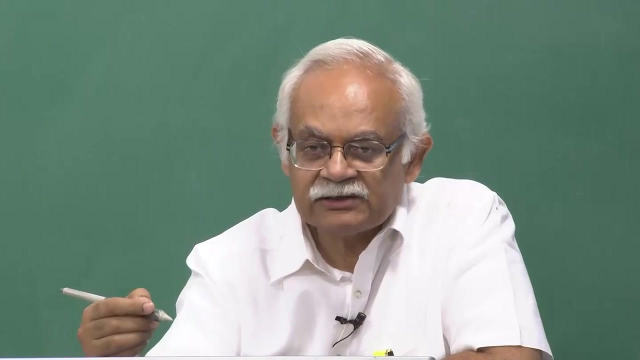 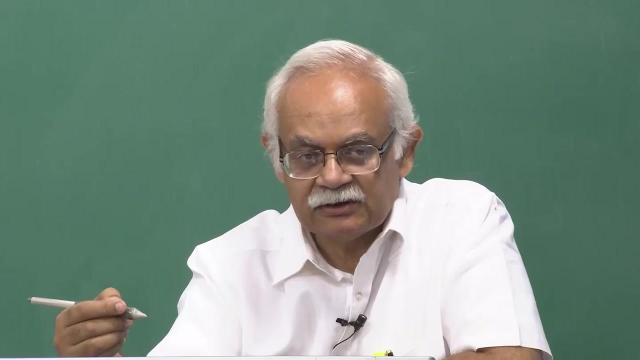 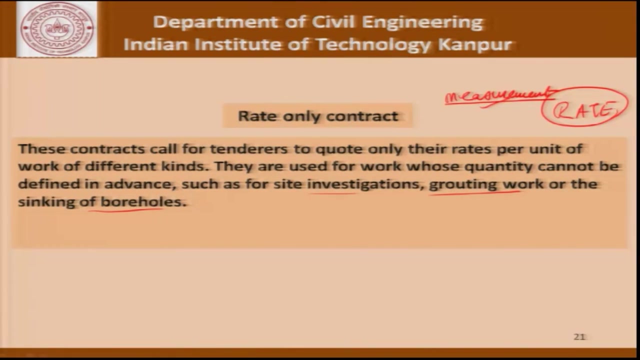